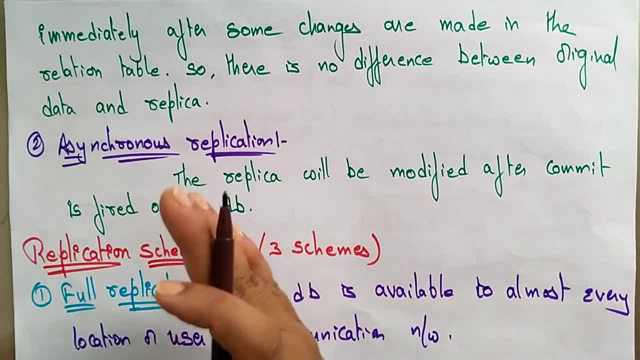 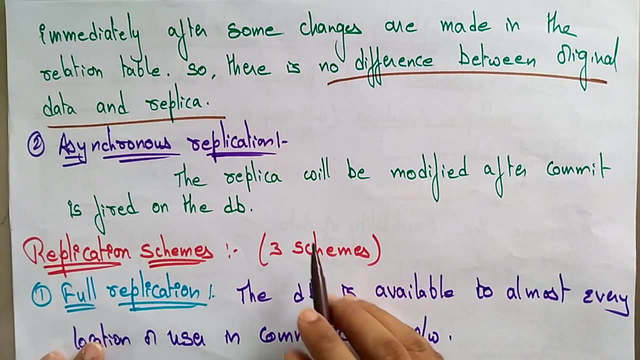 replica data in synchronous manner. so in the synchronous there are two different types of uh replications. one is a synchronous replication, another is asynchronous- in this synchronous difference between the original data and replica data. but whereas an asynchronous replication, the replica will be modified after commit is fired on the database. so 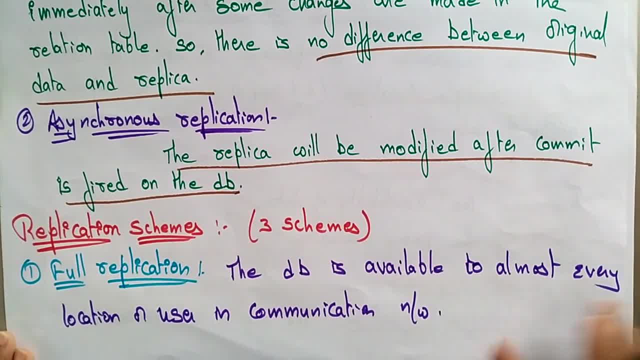 these are the two different types of the replications in database. now let's see the different schemes of replications. there are total three schemes that are present. the first one is a full replication. the name itself is saying it is a full replication. here the database is available to almost every location. 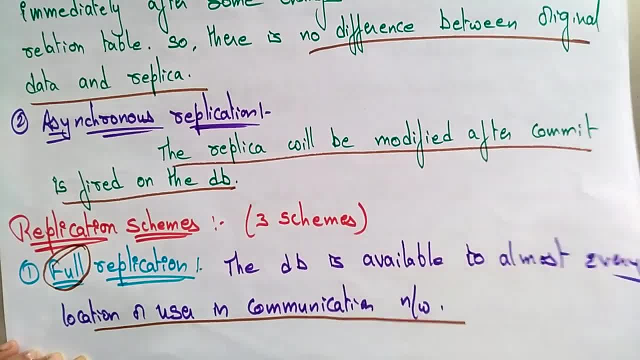 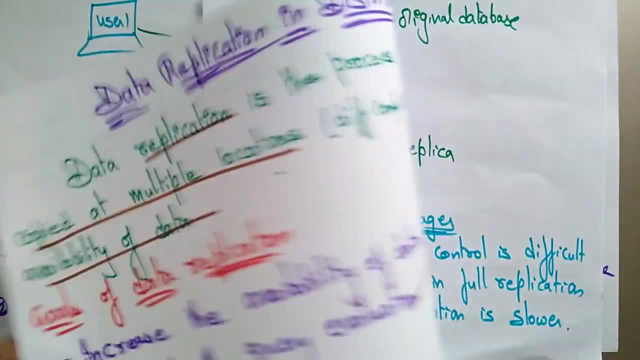 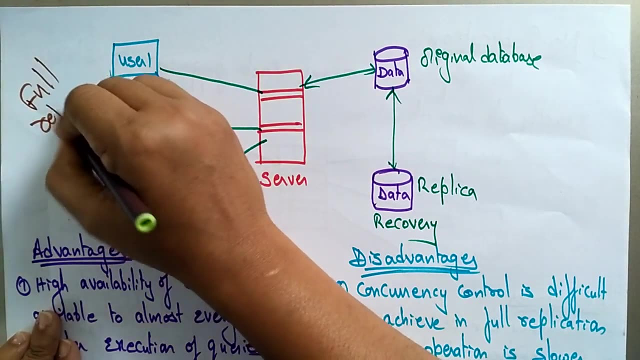 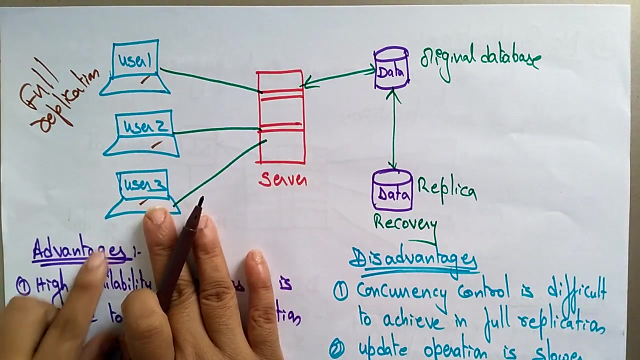 so user in communication network. okay, so here the database is available to almost every location. so that's why we call it as a full replica. did you see here in this example the full replication? it's a full replication. so here I have taken two, three server server user one, user two, user three and 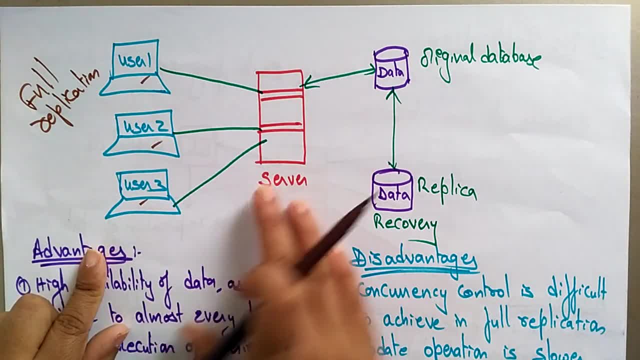 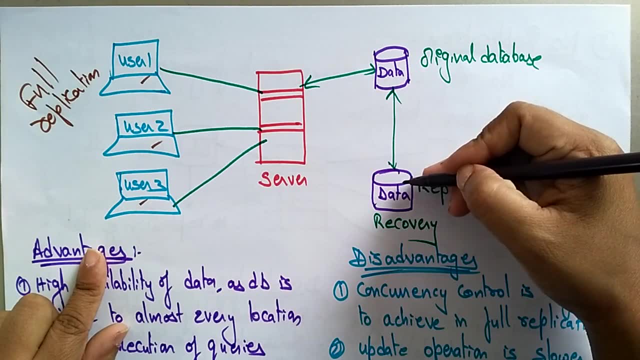 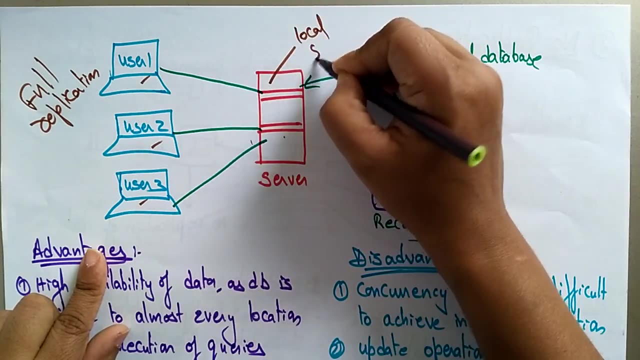 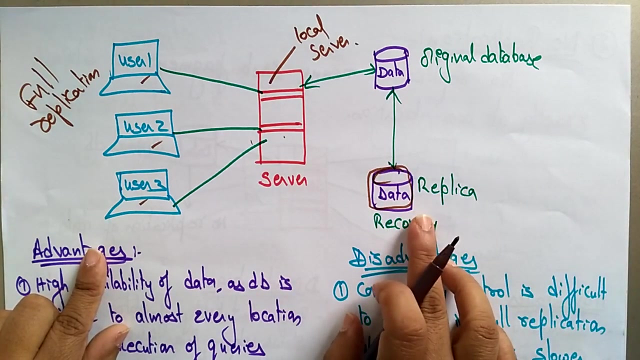 these users are connected to a server and this server is having a data which is a original database, is placed in this server. so again, there is one more data is placed on this server as a server is having. the main server is having some local servers. each local server is holding one replica data. replica database will be stored in. 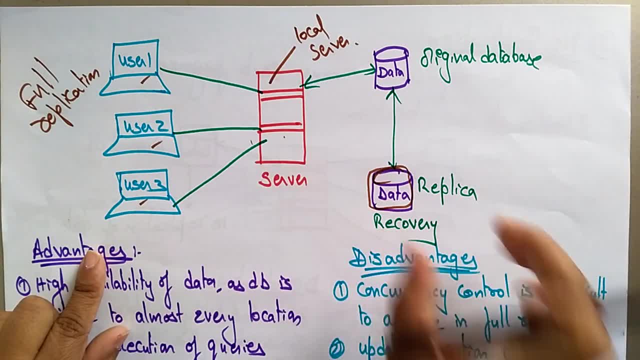 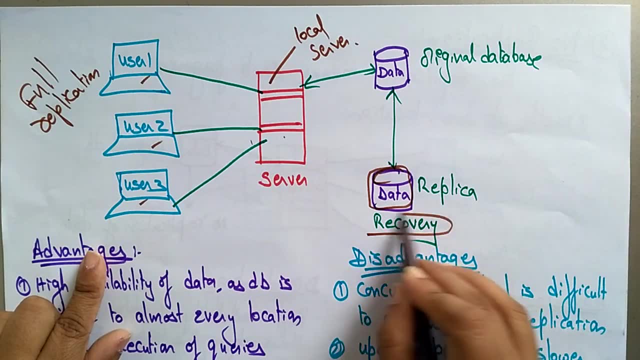 different local servers. so this is a replica. so whenever some data is lost, that is the original data. or some other data is lost in one local server to the server. if this replica data is going to recover that, okay, it sends that same information to this versional database so that this is a full replica. 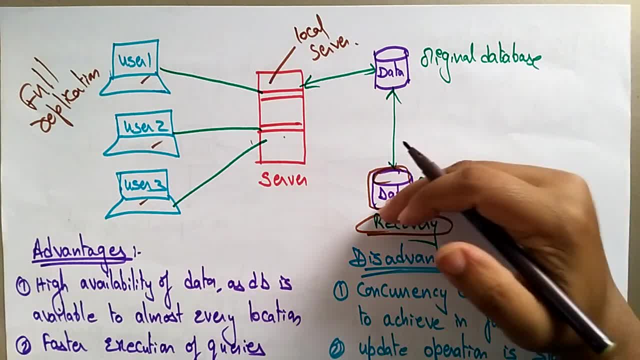 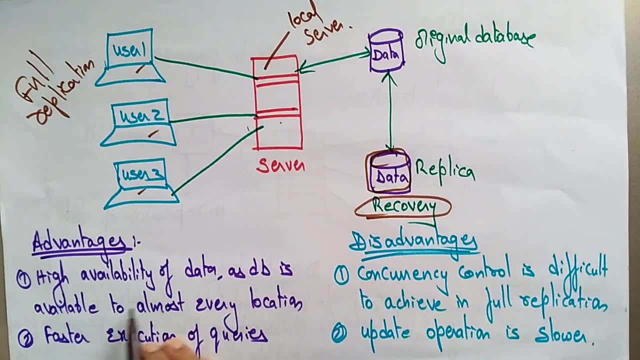 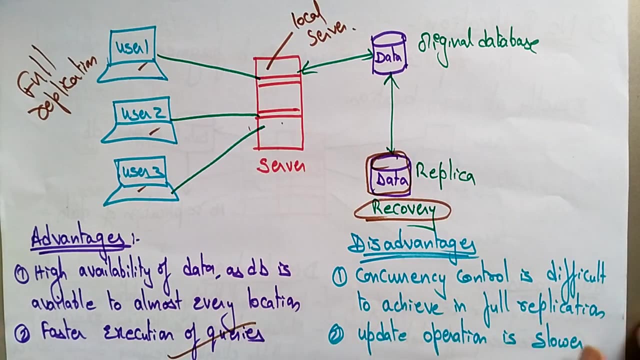 okay, even though one part, one concept decision, the complete data is going to be recovered, so this is a full replica. the advantages of the full replica is high availability of data, as database is available to a more almost every location, and it is faster execution of of queries. and whatever the disadvantages here, the concurrency control is difficult to achieve. 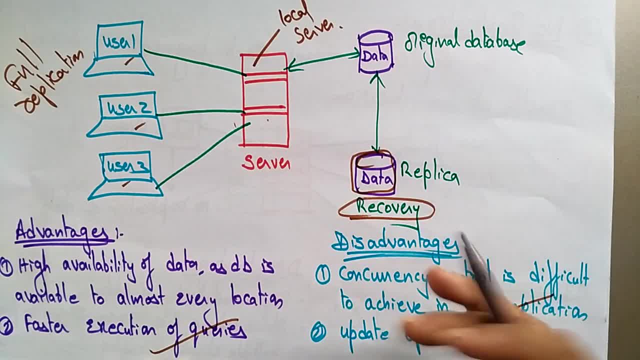 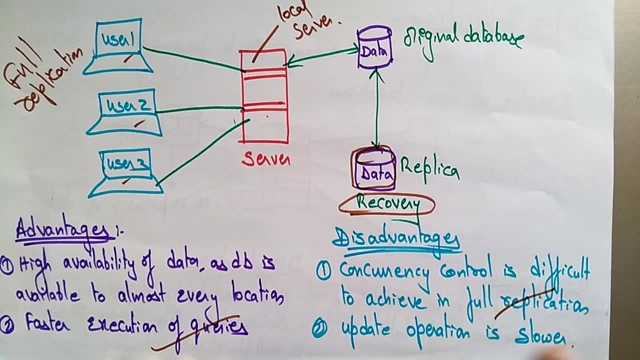 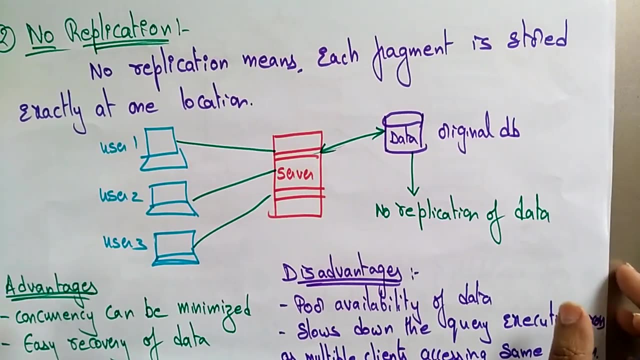 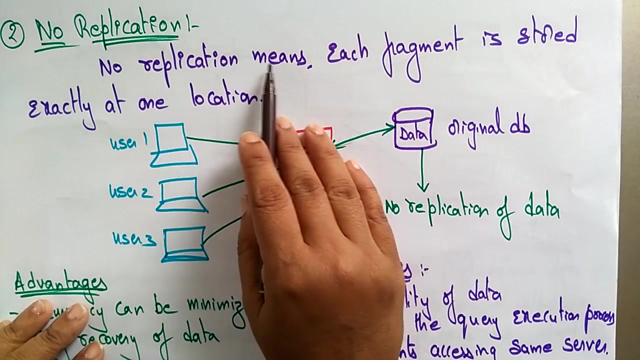 in full replication. so here it's because it's of having the replica, the complete information, the concurrency control is difficult to achieve. full replica and update operation is somewhat slower. and another type of replication schemes is: next scheme is no replication. no replication means there is no copy of the data is present. no replication means each fragment is stored. 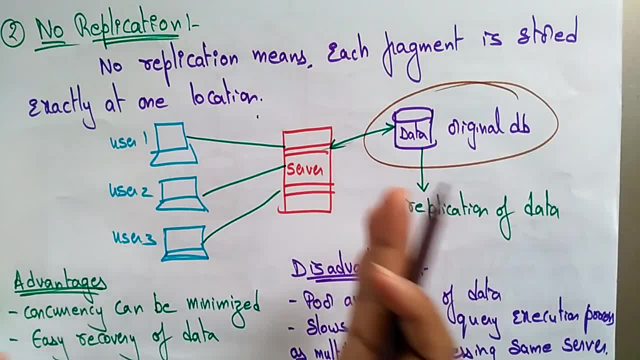 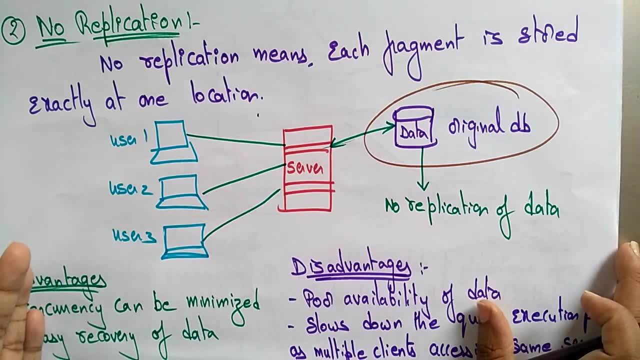 exactly at one location, so that is in only in one database. the original database is stored in the main server only, so there is no. I am not maintaining any replication to that database. so suppose if the database is crashed, there is no use means I can't recover that data. 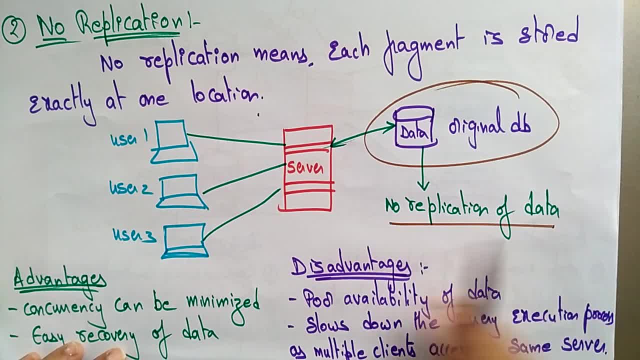 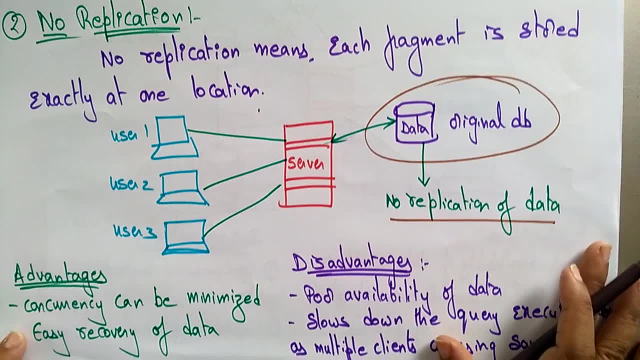 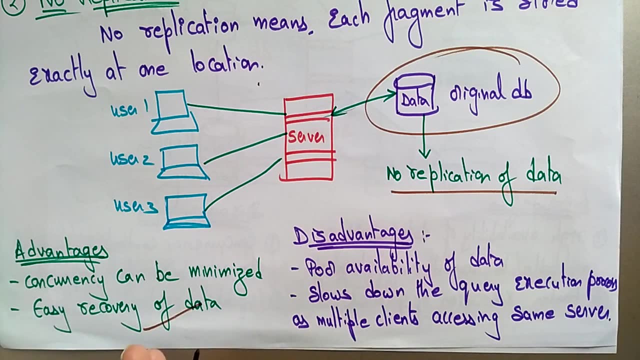 because I didn't save any replica data. no replication of data, okay. so no replication means only each. each fragment is stored in one location, so that is in only in one database. fragment is stored exactly at one location only, and the advantages here is concurrency can be minimized and easy recovery of data. so here the thing is. i said no replication of data means 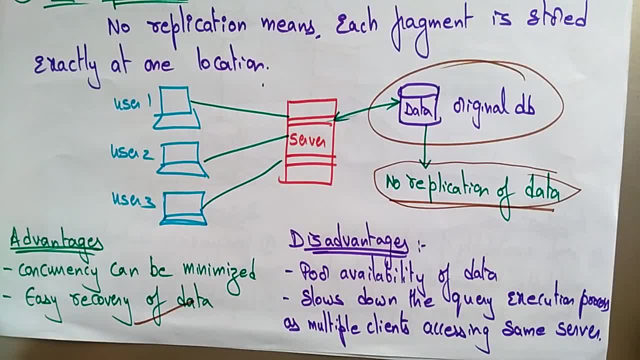 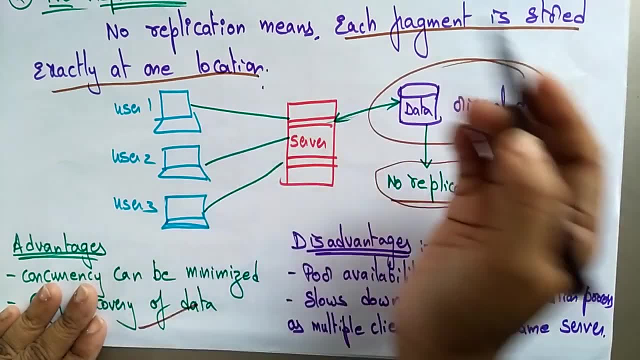 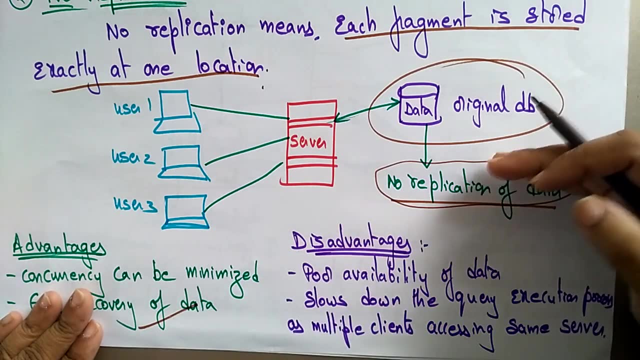 whenever the data is lost. we can't recover that, but here in no replication means each fragment is stored exactly at one location. okay, so the complete query is divided into different parts. okay, each part is sending to one location, exactly to one location. all the data will be gathered. so 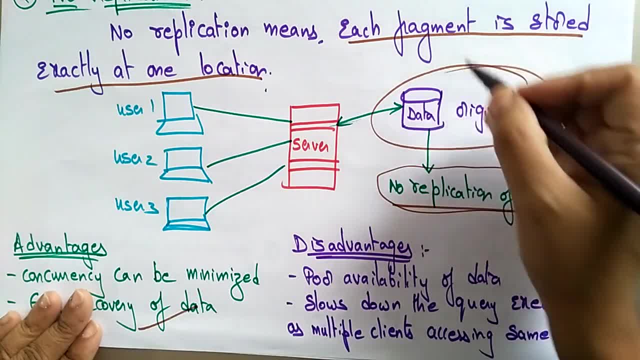 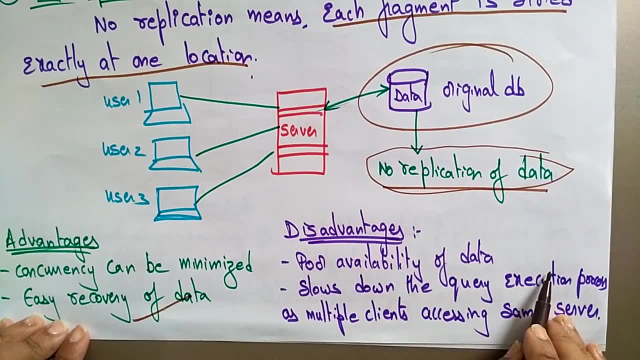 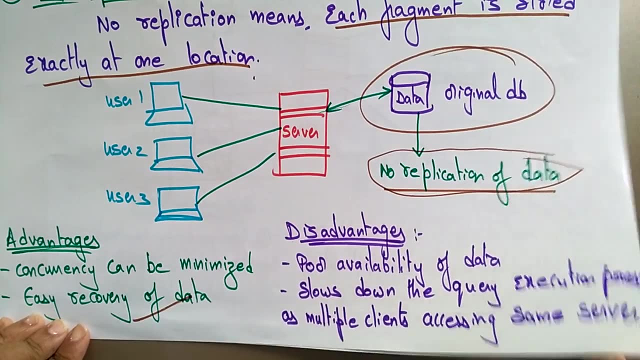 that is, a original database will be gathered. so for each fragmentation we are not storing the replication of data. okay, and the disadvantage is poor availability of the data and slowdowns the query execution process as multiple clients accessing the same server and another replication schema is partial replication, the partial replication. 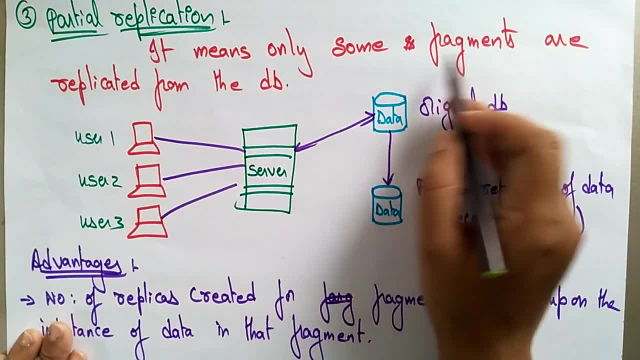 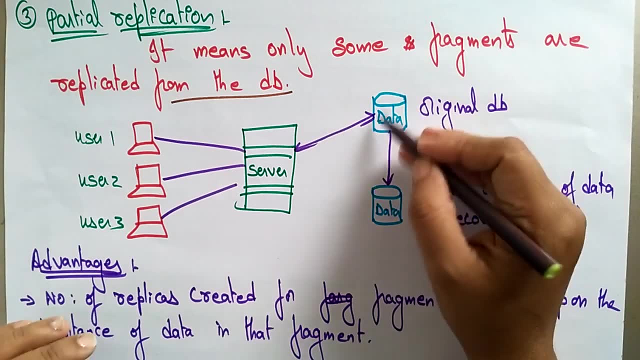 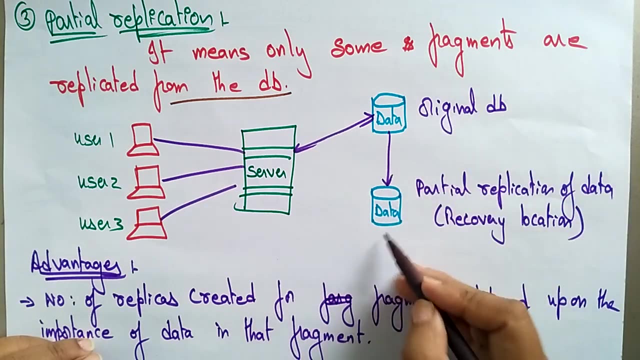 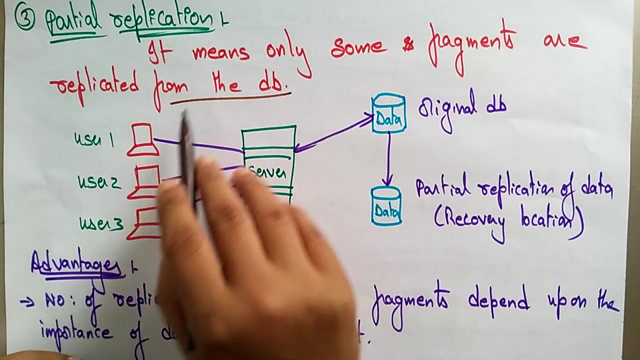 means here it means only one, some, only some fragments are replicated from database, not the all, only some fragments. so here in the database you are having one complete database and this database is divided into different fragments. so here in the partial replication of data, also it divided into fragments. so here the partial replication it means only some fragments are.